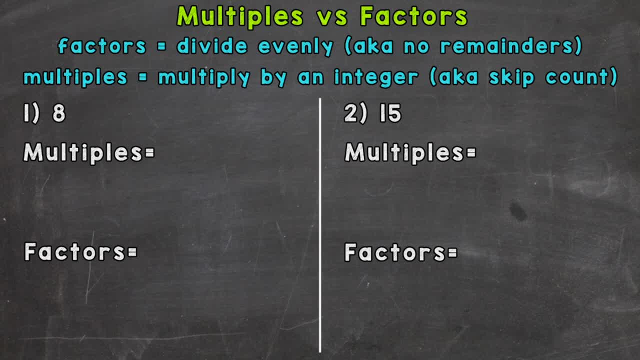 have eight And we'll start with multiples, So we need to list some multiples of eight. Now, multiples are the result of multiplying the given number by integers, so no fractions or decimals, And we can think of this as skip counting. Let's make sense of that by writing. 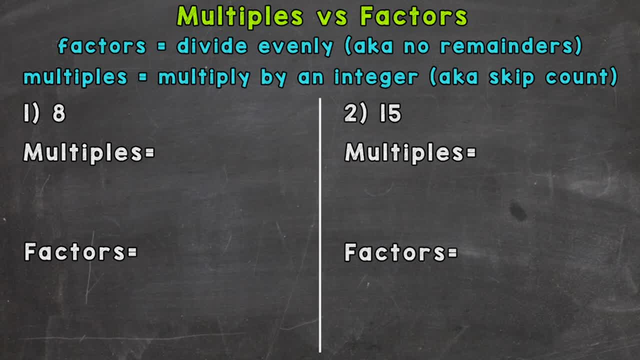 out some examples here, So the multiples of eight. we can start with eight. Eight times one equals eight. So we multiplied eight by the integer of one. Now we can multiply by the integer of two. So eight times two is 16.. 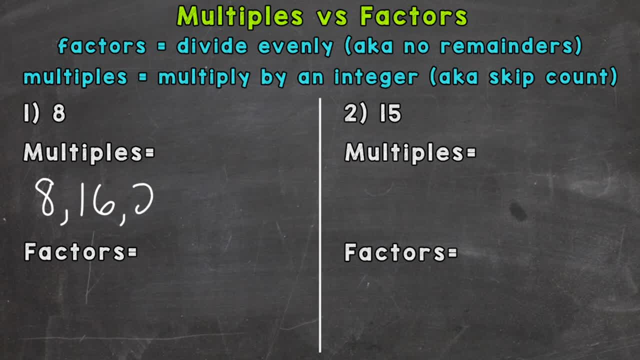 Then three. Eight times three is 24.. And you can see how this is turning into just counting by eights, or skip counting. Eight times four is 32.. Eight times five is 40. And so on and so forth. So those multiples will continue on forever. So it's all the numbers that eight will hit. 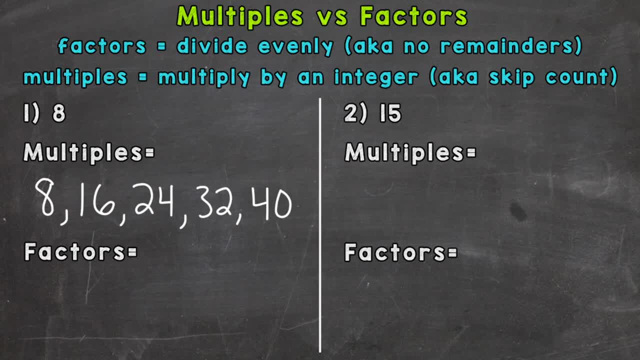 if we count up by eight, Or think of it as we multiplied eight by integers, starting with one, So we multiplied eight by one, And so on and so forth. So those multiples one, And then going two, three, four, five, six, seven, eight, And again it goes on forever. 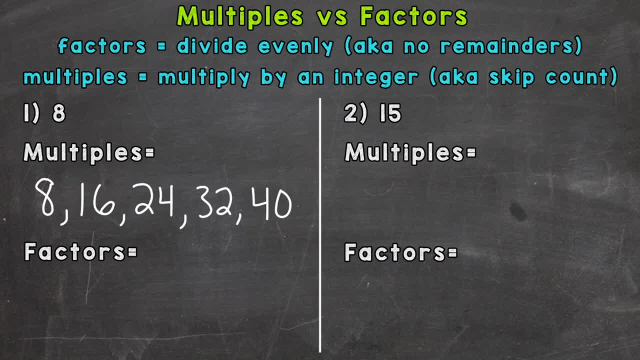 Now. multiples can be positive and go up in value, or multiples can decrease in value. There are negative multiples, but we are only going to be working with positives in this video, So let's move on to factors, And factors are all of the numbers that the given number can be. 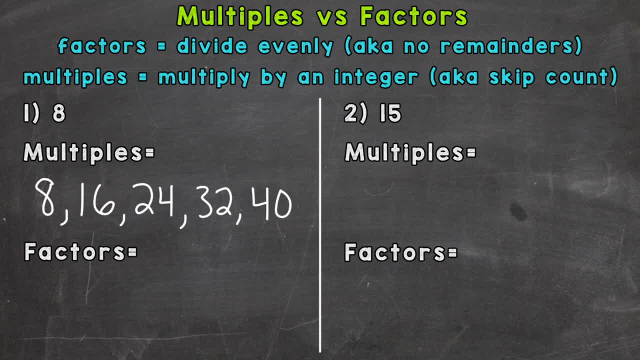 divided by evenly, So no remainders. Or you can think of factors as the numbers that can be multiplied in order to get that given number. Factors are numbers that are multiplied to get a product. I like to think of factors as all the numbers that can go into a 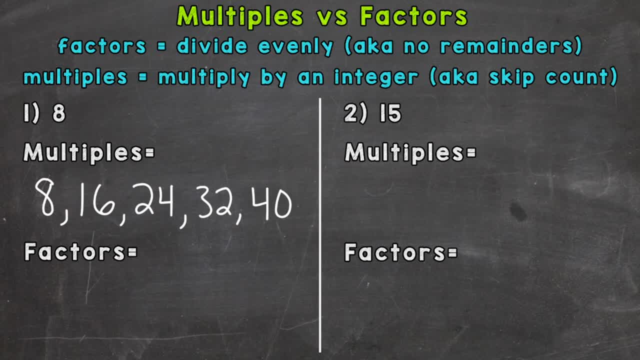 given number. That's not the most mathematical or technical way of thinking about it, but it can help with determining the difference between multiples and factors. So let's find all the factors of eight, And when we find factors, I like to start with two numbers, and then I'm going to. 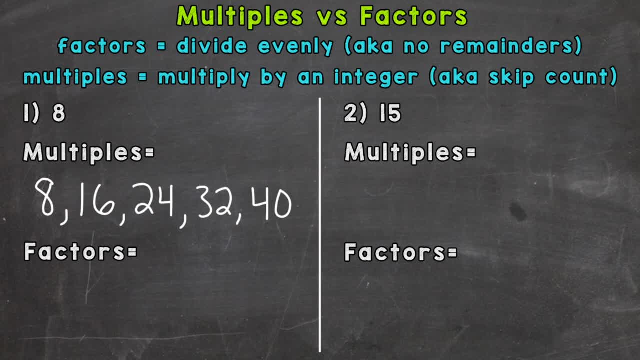 find two numbers for two factors for every number, And those factors are one and then the number itself. So one and eight. I can do eight divided by one and that will divide evenly- I will not get a remainder. And I can do eight divided by eight, Or you can think of it as one times eight. 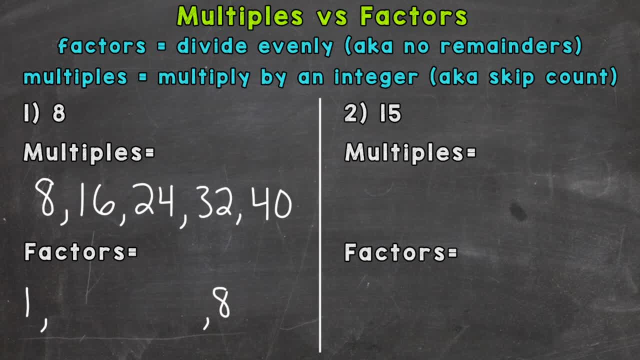 equals eight. So all the math facts, all the multiplication facts, that will equal eight, And we can think of this as a factor pair Here. So we'll start with one and eight, And for some numbers those are the only factors. 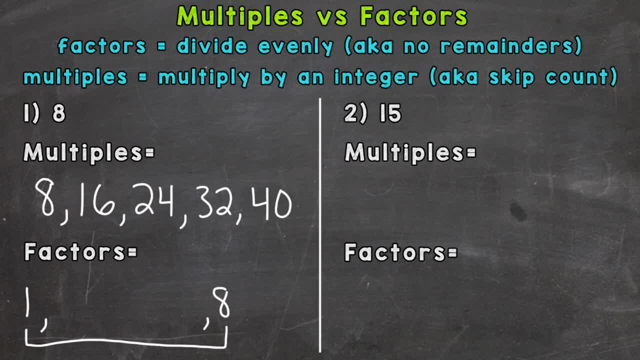 one and the number itself. Those numbers are called prime numbers. But eight is composite, so it has other factors involved here. So what other numbers can go into eight? you can think of it as or a multiplication fact to equal that given number of eight. 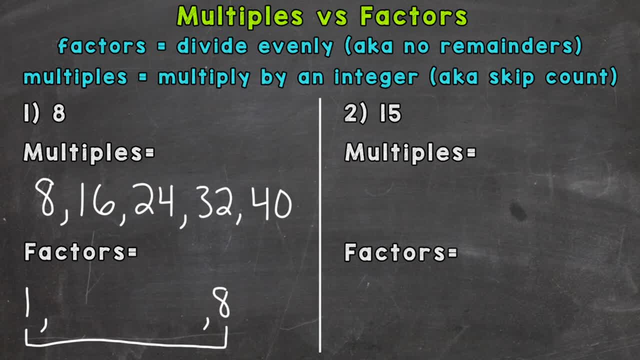 Well, I could do eight divided by two. right Two can go into eight. So that's my next factor. And I know two's partner is four, because eight divided by two equals four. Or I could do eight divided by four equals two. Or think of it as two times four equals eight. So different ways of 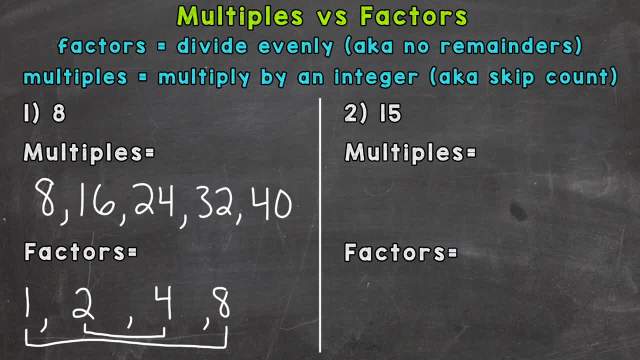 thinking about factors, but it's all the numbers that can divide evenly, aka no remainders as far as eight goes. Now, when I wrote my factors list, I put one and eight and then I put a big gap in the middle, And then I put one in eight and then I put a big gap in the middle. So I put 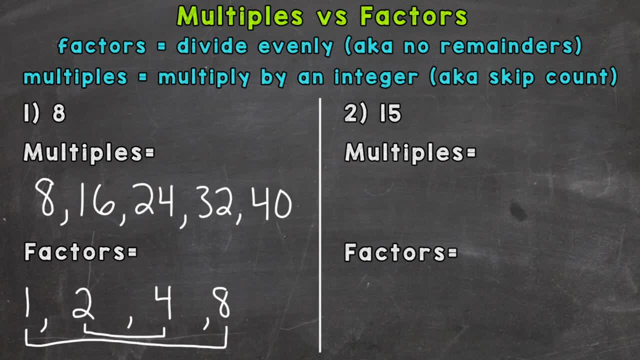 a big gap in the middle And then I put one in eight and then I put a big gap in the middle, middle there. That way I can fit any other factors. that would be between 1 and 8 and they would all go in order. You'll get better with spacing the more. 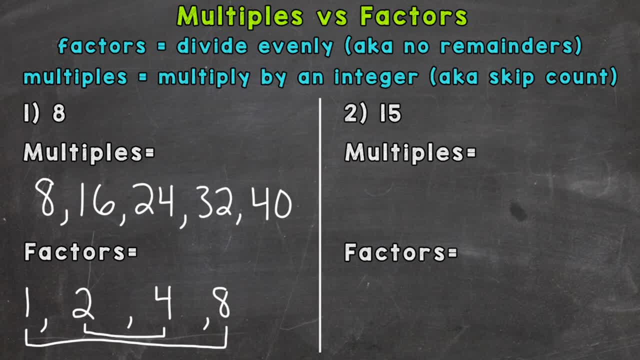 you do. of those, Let's go to number 2 and write out the multiples of 15.. So we'll start with 15 times 1, or just start with 15 and skip count, however you like to think about this. 15 times 2, 30.. 3 is 45.. 4 is 60.. 5 is 75.. And again, those do. 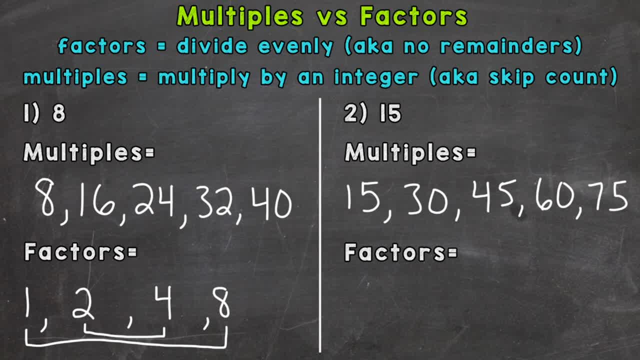 continue on forever, but we'll cut it off right there. As far as factors remember, we start with 1 and the number itself, because 1 can go into 15 and then 15 can go into 15.. I like to leave a little gap there that way, if there are any other. 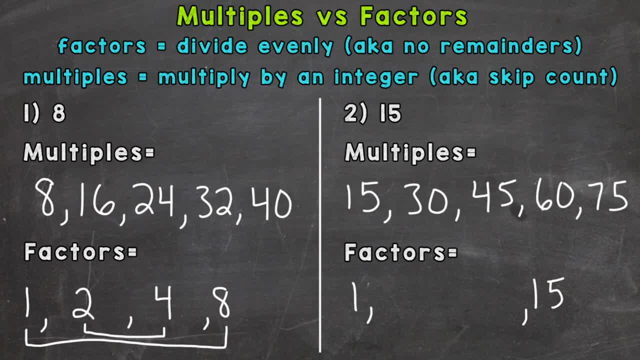 factors. I'm not going to be able to do that, So I'm just going to go ahead and I can list them in between 1 and 15 and they're all in order. So think about 15.. What other numbers go into 15 or can multiply to get 15?? Well, I know 15. 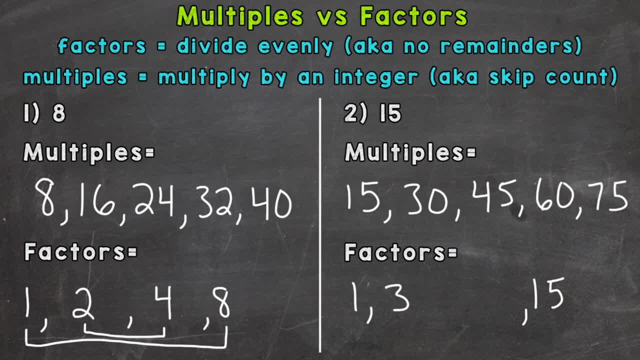 divided by 3 and 3's partner is 5, right, Because, let me start with this- 1 and 15 are partners, and then 3 and 5 are factor pairs or partners, And those are all the factors of 15.. 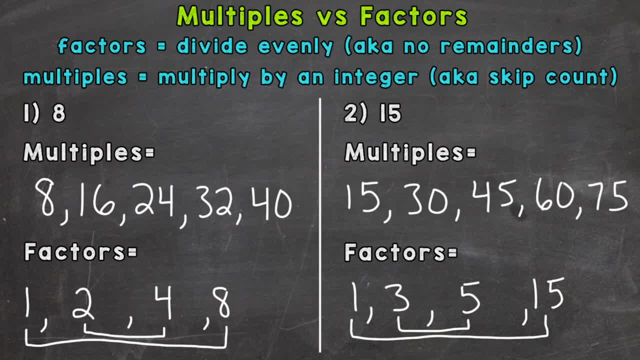 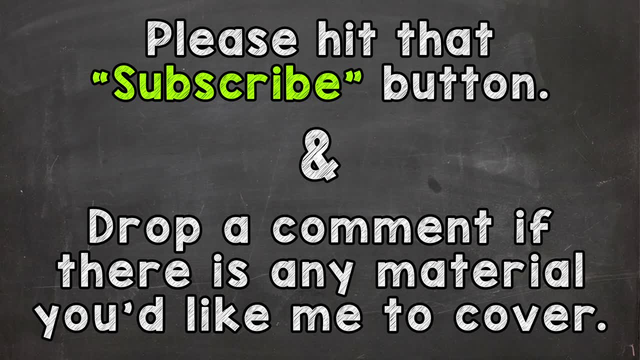 So there you have it. There's the difference between multiples and factors. I hope that helped. Thanks so much for watching, Until next time, peace. 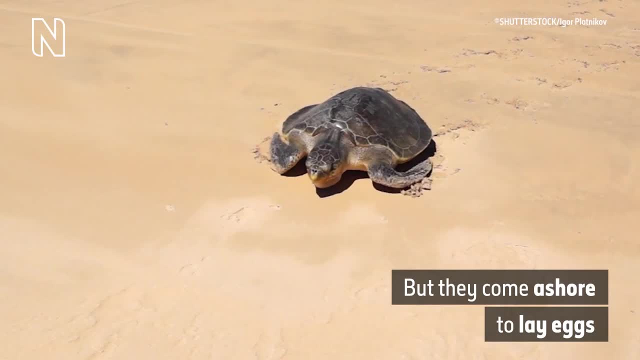 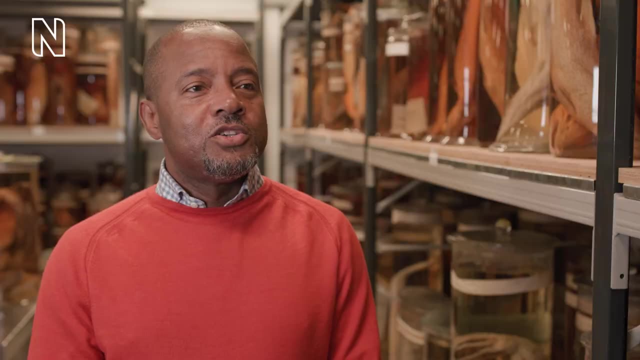 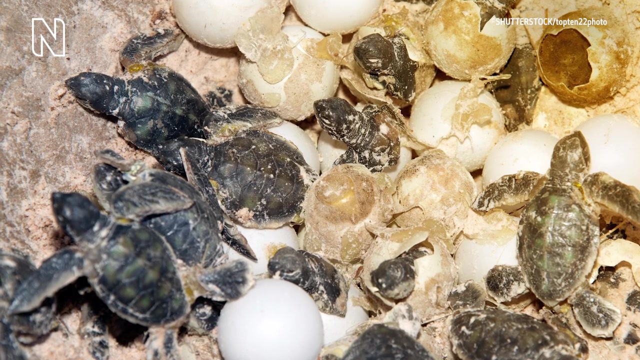 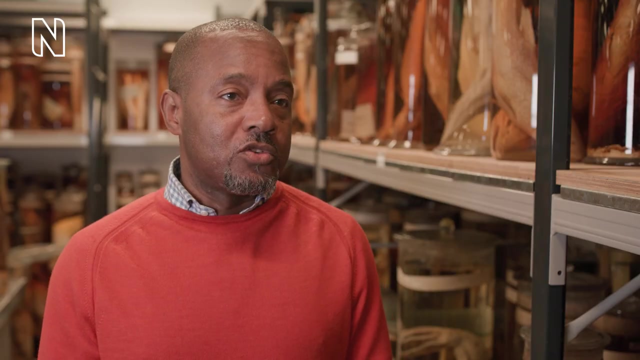 Sea turtle eggs are laid in clutches in the sand on beaches. The temperature of the sand and surrounding environment affects the sex of the turtle that eventually hatches. A warmer environment leads to females, while a cooler one leads to more males and is called temperature. 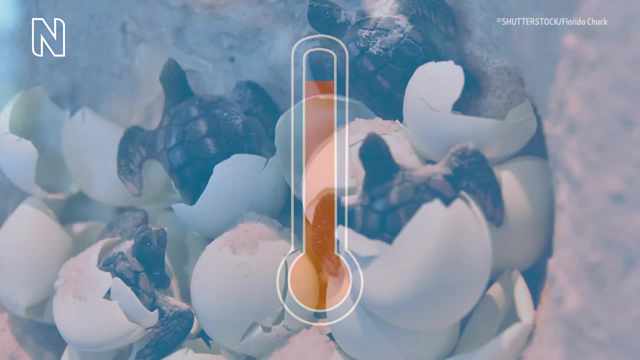 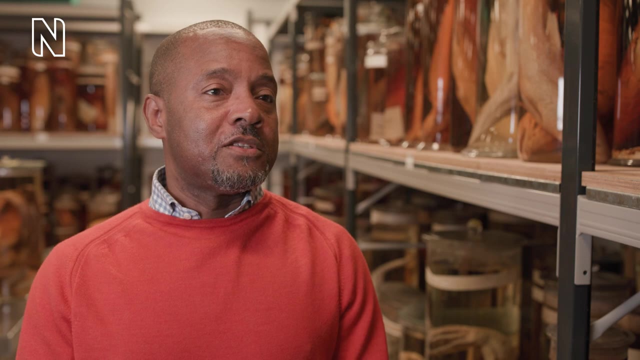 dependent sex determination. A difference of only a few degrees can change the sex of an entire clutch of eggs. Global warming is putting the future of many turtles at risk. as the world heats up, It follows that fewer males are being born in relation to females. 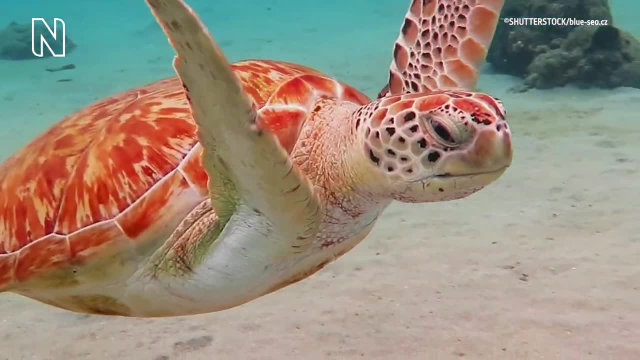 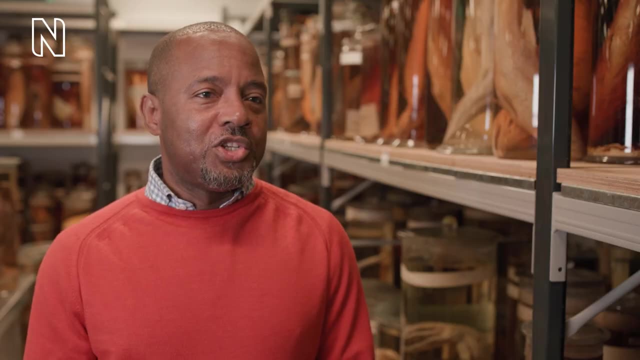 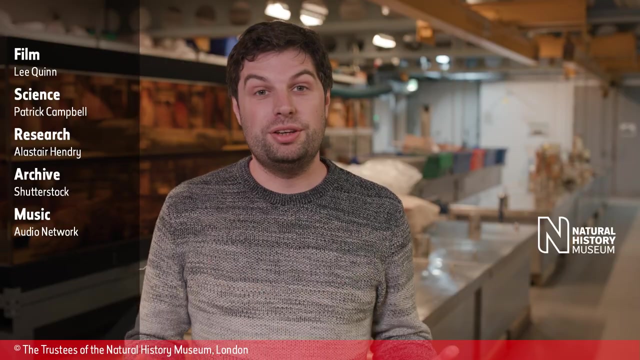 When those females reach maturity, they may struggle to find a mate, and the species could very well and very quickly see their populations crash. Turtles have survived climate change before, but the speed of change we are experiencing now may prove too much for them. Thank you for watching everyone. hope you enjoyed that. 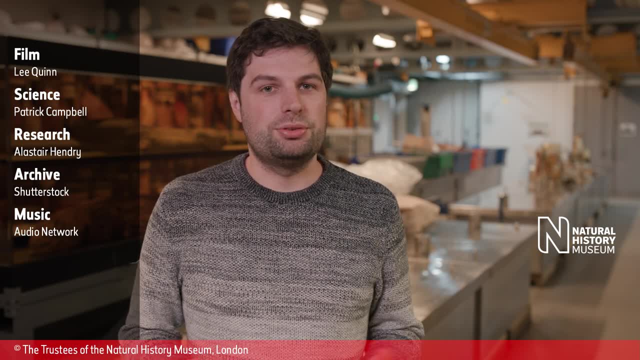 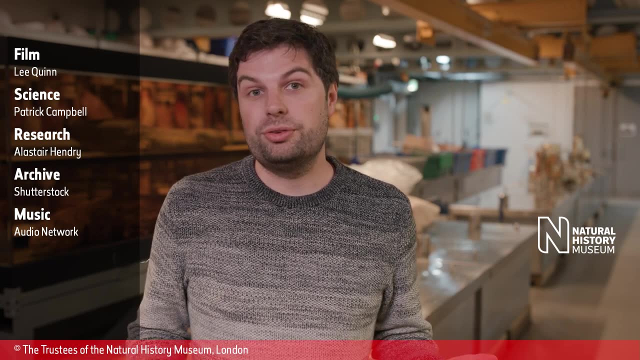 We were just learning there how turtles can be affected by changes in temperature, and it's one of the many surprising effects that a changing climate can have on our world and the species in it. If you've got any thoughts on that and want to share it with us, please,